dependent on the magnitude of the current in the power lines. Power loss due to resistive heat production is dependent on the magnitude of the current in the power lines. Power loss due to resistive heat production is dependent on the magnitude of the current in the power lines. 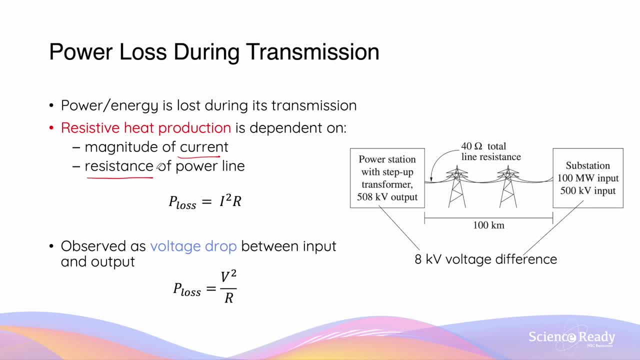 And the resistance of the power line itself. Specifically, power loss can be calculated by using this equation: Power loss equals to I squared current squared times. where R, where R is the resistance of the power line in ohms. As a result of the power loss, there's always a voltage difference between the source. 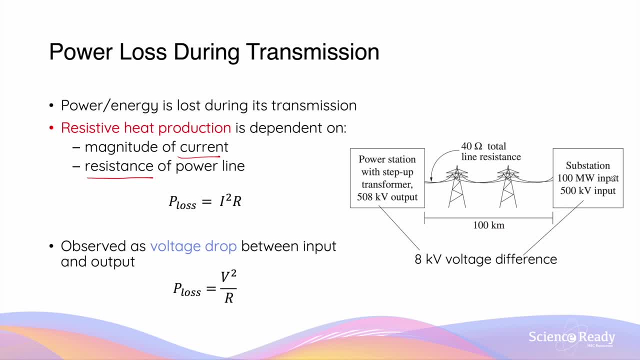 and the destination of the power. In this case, this is the power between the power station which produces the energy and the substation which receives the energy. This difference in voltage is often referred to as a voltage drop. When there's a larger voltage drop, 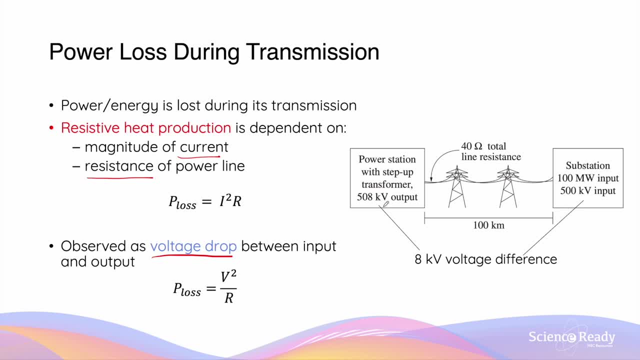 there is a larger amount of energy lost during transmission. We can also use the voltage drop to calculate power loss, where power loss is equal to the square of the difference in voltage between the power station and the substation. So this is our voltage drop divided by the resistance. 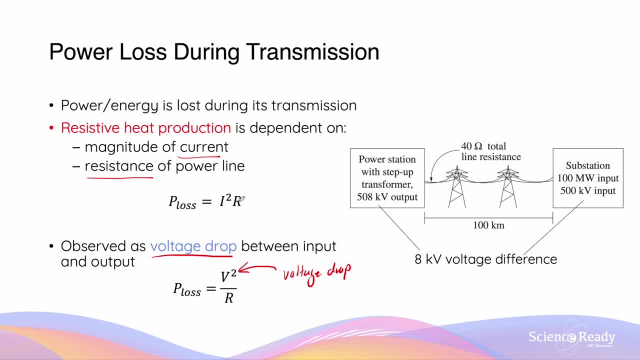 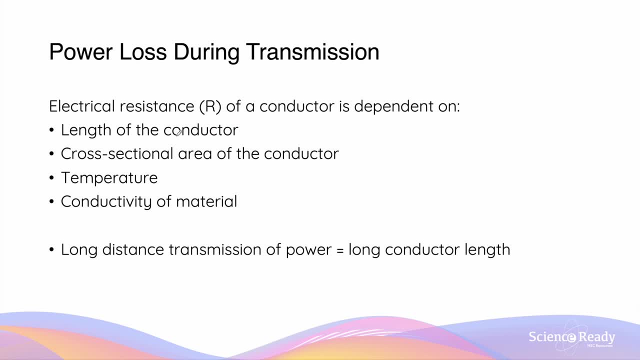 of the power line. You can use either of the two equations, depending on whether you know the current flowing through the power line or the voltage drop that's observed due to the power loss. By way of review, the electrical resistance R of a conductor is dependent on various factors. 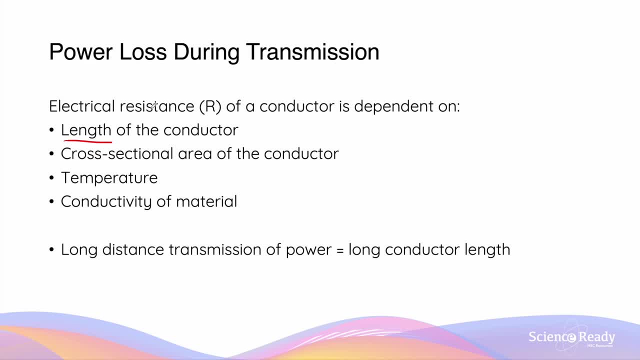 This includes the length of the conductor. the longer the conductor, the higher the resistance it has. It depends on the cross-sectional area of the conductor. Figure the cross-sectional area, that is, the thickness of the conductor and the resistance of the conductor. 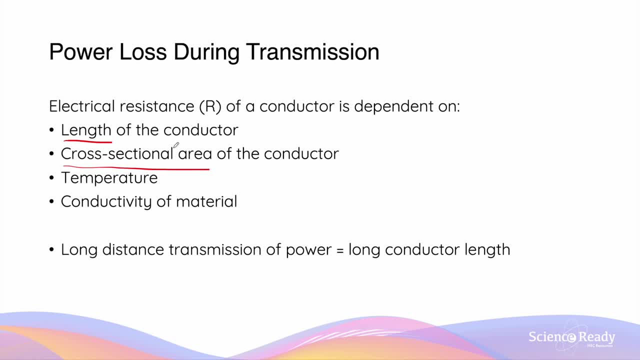 Thicker the wire, lower the resistance it has. The temperature for metals, higher the temperature, higher the resistance And also the conductivity or the intrinsic resistance of the material itself. Different materials, such as copper versus aluminium, although they can both conduct electricity, they have different degrees of electrical resistance. 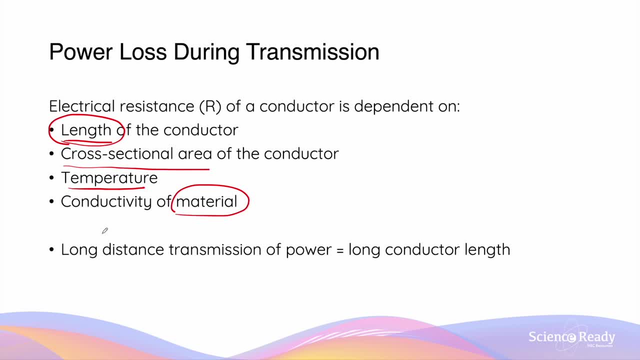 We want to focus on the first factor, that is, the length of the conductor, because, as we discussed earlier, most power stations are located in remote regions, quite far away from metropolitan areas which will receive the power. Long distance transmission of power is associated. 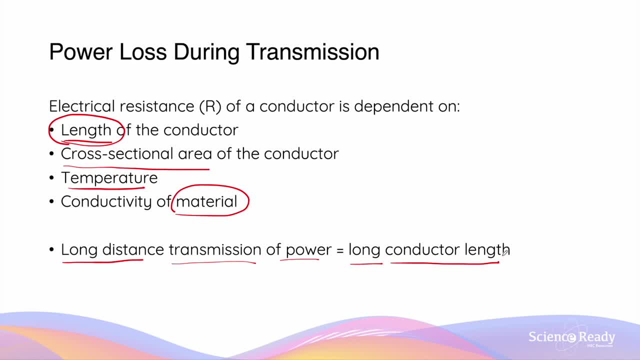 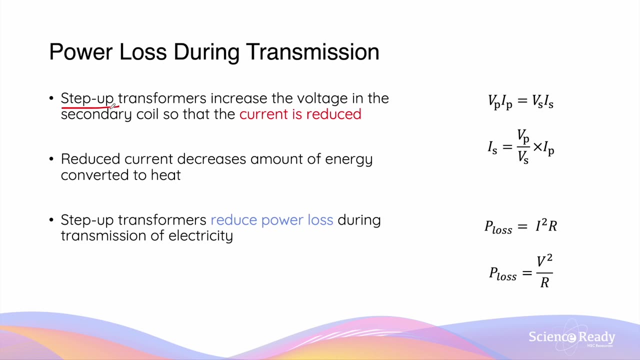 with a very long conductor length, which means the resistance of the transmission line is greatly increased due to the long distance it has to traverse. The inevitable power loss due to long distance transmission is where step-up transformations occur. This is where step-up transformers come into play. A step-up transformer increases the voltage in its secondary coils. 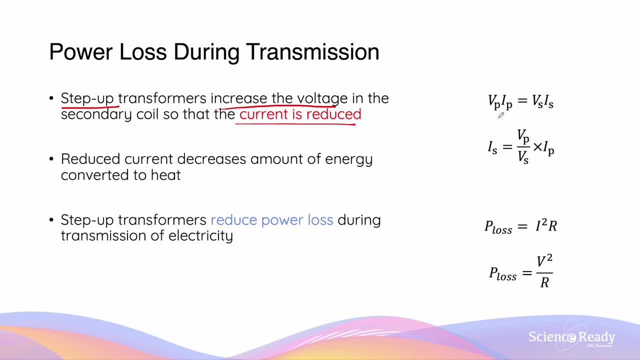 and decreases the currents that flow through them. By way of review for an ideal transformer, the electrical power input in the primary coils equals to the power output in the secondary coils. So if we increase the voltage across the secondary coils by using a step-up transformer, 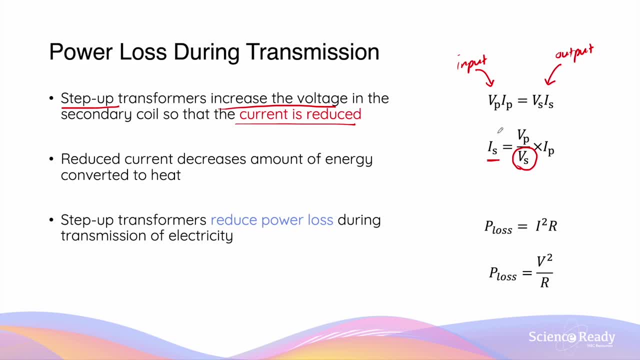 the current that's flowing through the secondary coils, that is, the output of the transformer, will be greatly reduced, because the secondary current is inversely proportional to the secondary voltage. And by reducing the current, the amount of energy that's converted into unwanted heat is decreased during transmission, because the power loss over 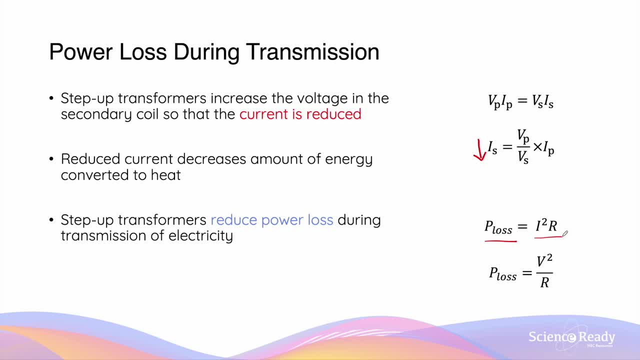 the power line is given by I squared R, where I is the current flowing through the transmission line after it has gone through the transformer. Therefore, step-up transformers reduce power loss by decreasing the magnitude of current through the transmission power line. Alternatively, we can also use a second equation. 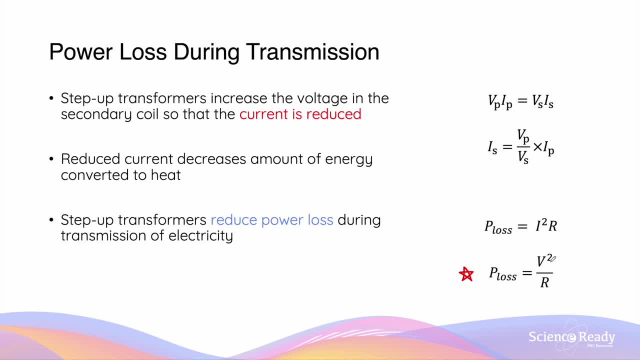 where power loss equals to the voltage drop squared above the resistance. When we have a smaller current, there's less power loss, and this is usually associated with a smaller voltage drop. It's important to distinguish between a smaller current and a smaller voltage drop. 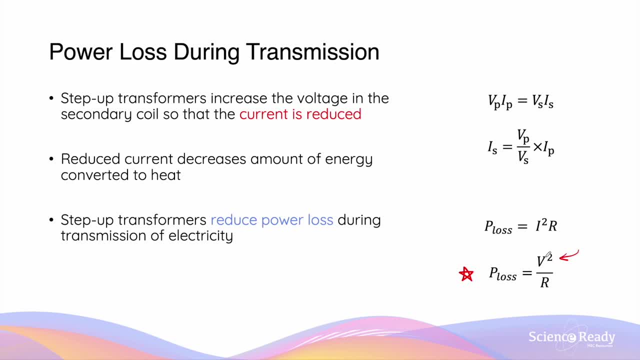 We can distinguish that this V squared. it is not the same voltage as the secondary voltage in my first equation. So although a step-up transformer increases the voltage, this is not the same voltage. we need to substitute for the power loss formula. The V squared in this equation refers to the voltage drop. That is the difference in voltage. 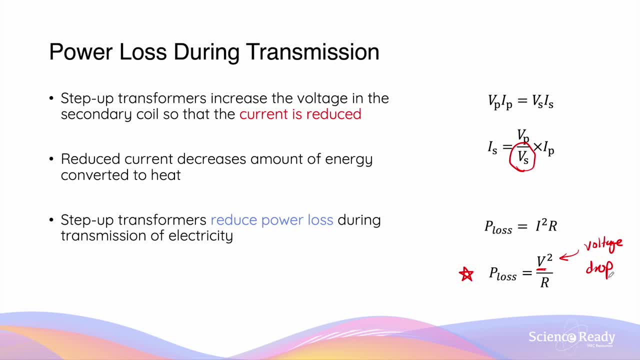 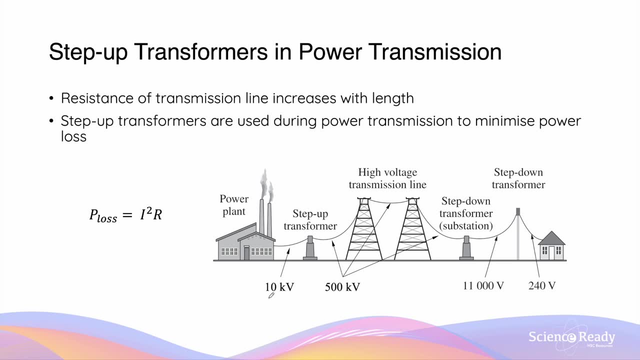 between the power station and the destination which receives the power. Let's look at a specific example. The power output of a power station has a voltage of 10 kilovolts, that is, 10,000 volts. Before this electrical energy of 10,000 volts is transmitted, a step-up transformer is used. 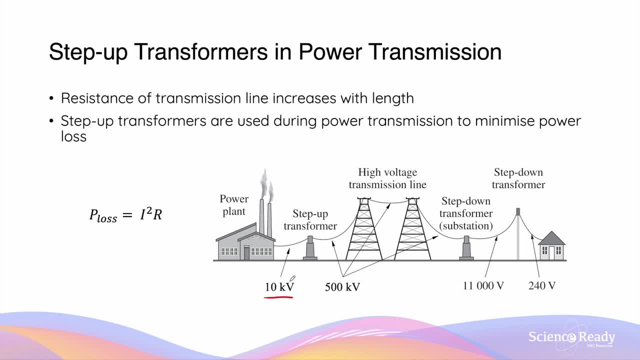 to greatly increase the voltage from 10,000 volts to 500,000 volts. When the voltage is increased, the magnitude of current that's flowing through the transmission wire is greatly reduced. This is usually reduced by the same factor, That is, if the voltage here is increased by 50 times. 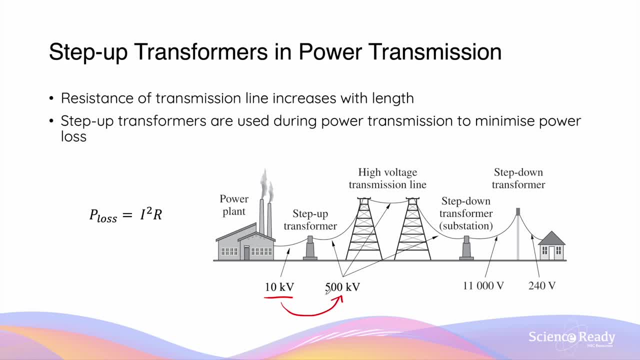 the current going through the wire will also decrease by approximately 50 times as well, Since the power loss going through the transmission line is proportional to the square of the current flowing through it. when the current is reduced, the amount of energy that's transformed into heat, as the current is flowing through the high voltage transmission line. 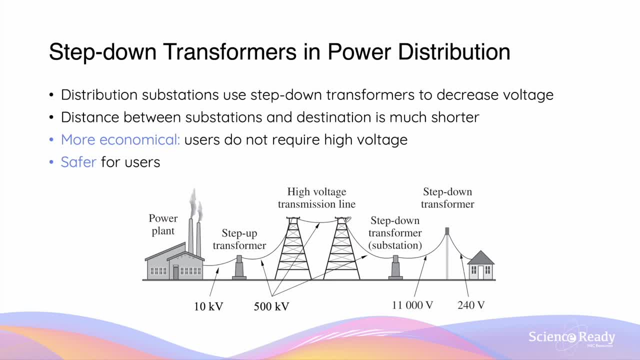 is greatly reduced After electricity is transmitted over a long distance and finally reaches a substation that is much closer to the user of this energy. a step-down transformer is used to decrease the voltage, Since the distance between the substation and the final destination where the energy will be used is much shorter compared to the distance 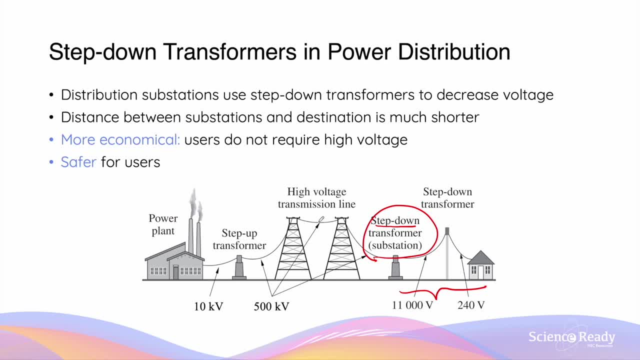 that needs to be traversed during the transmission stage. we no longer require high voltage, as the resistance of the wires are much smaller compared to before At the substation. decreasing the voltage is also more economical, as the end users, such as our households, do not require the high voltage that was used for transmission. 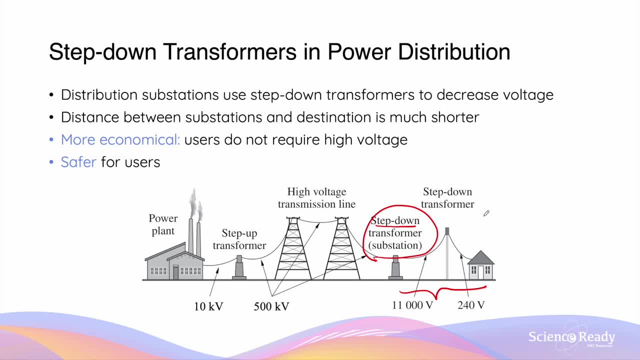 Right before the electrical energy is delivered to our households, another step-down transformer is usually used to further decrease the voltage to a safe value, usually 240 volts. The low voltage during the distribution of power and its use in homes is much safer compared to the high voltage used during transmission, Both step-up and step-down.